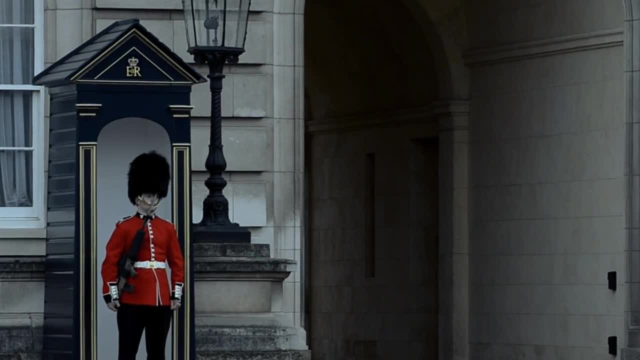 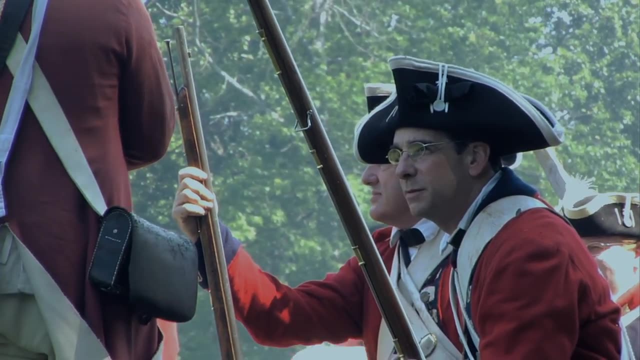 a time when the United States didn't officially exist and America was ruled by England. In fact, the separation of the Carolinas happened during that colonial period, in 1712 to be precise, with the one original Carolina colony splitting into the separate colonies of North. and South Carolina. In fact, the separation of the Carolinas happened during that colonial period. In fact, the separation of the Carolinas happened during that colonial period, in 1712 to be precise, with the one original Carolina colony splitting into the separate colonies of North and South Carolina. 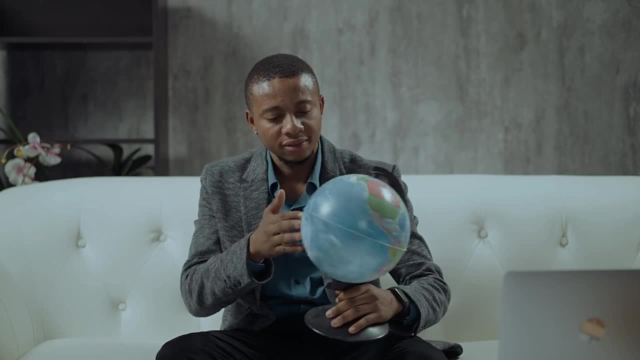 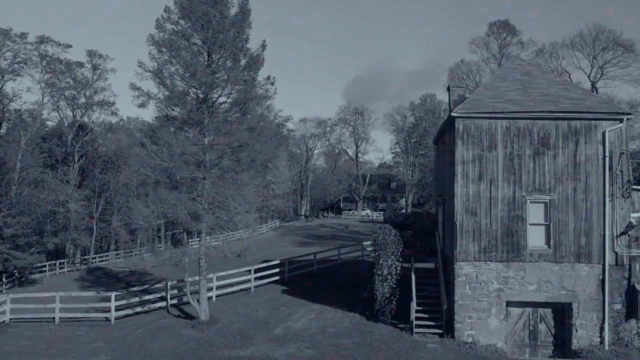 That colonial divorce, a result of contrasting differences from geography to international loyalties, was peaceful yet tenuous. Anyway, both Carolina colonies, separately but almost simultaneously, became part of the first group of 13 US states back in 1788.. 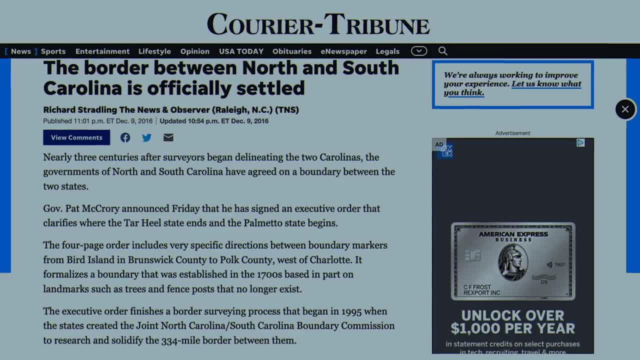 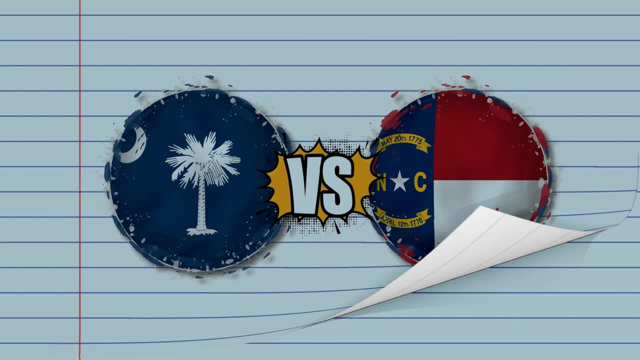 Now Carolinas may share a last name, a deep history and a border that took nearly three centuries to officially settle. However, they also share a historic rivalry, after centuries of competing for resources and residence and due to important cultural differences between the two, And I'm not just talking about the North. 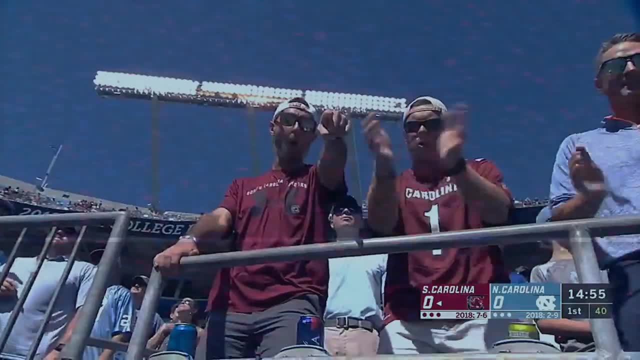 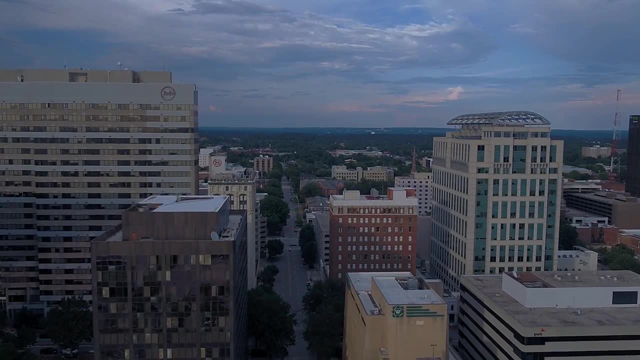 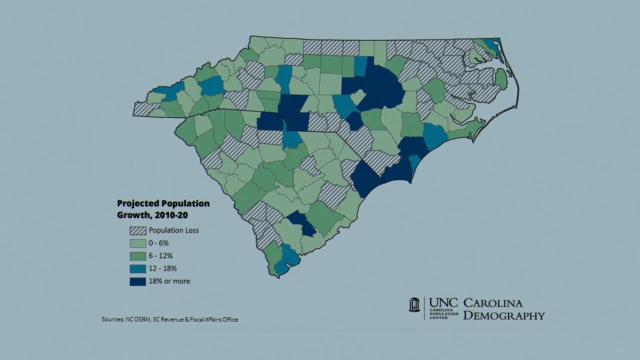 Carolina Tar Heels and South Carolina Gamecocks football competition here. So let's compare and contrast these distinctly different Carolina states, ultimately outlining which Carolina is the better state today: South Carolina or North Carolina. I know I already mentioned that North Carolina has a population that doubles South Carolina's. 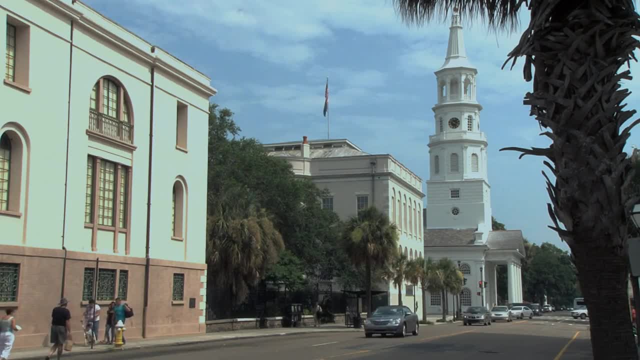 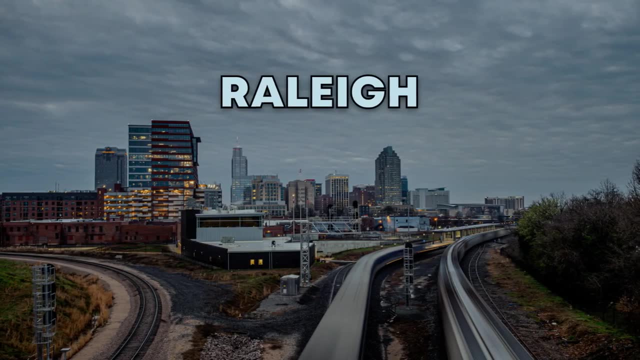 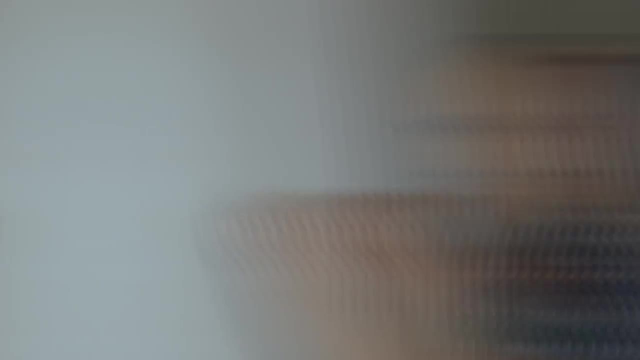 but I was actually a little surprised when looking at the size and scale of the three biggest cities in each of these states. The biggest cities in North Carolina are Charlotte, with 903,000 residents, Raleigh with 480,000 residents and Greensboro with 304,000 residents, While even the biggest city in South Carolina 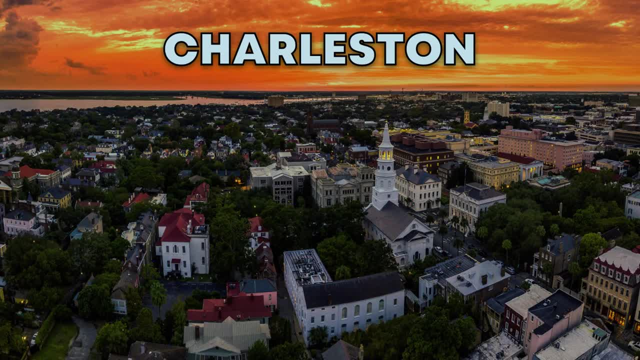 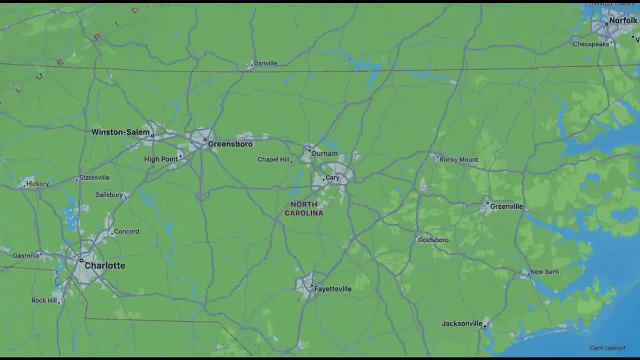 Charleston only has a population of 156,000 residents, Columbia has just 138,000, and Mount Pleasant has less than 100,000.. In fact, the seventh largest city in North Carolina, Cary, has more residents than Charleston, South Carolina's most populated city. It's a little different when you look at amenities and attractions, though, because while Charlotte is a real big city with an elite skyline and major economic opportunity, other Carolina cities on both sides of the Carolina border feel much smaller and perhaps a little more charming, Though, frankly, there are plenty of growing economic opportunities. 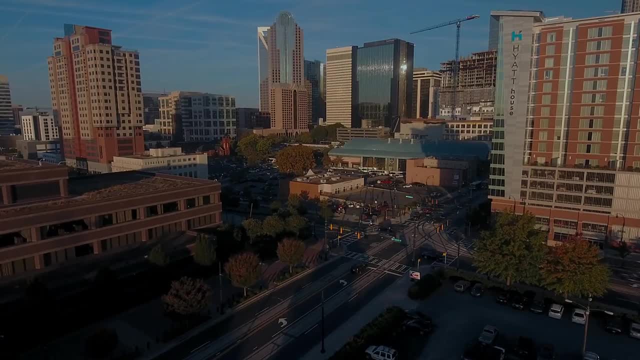 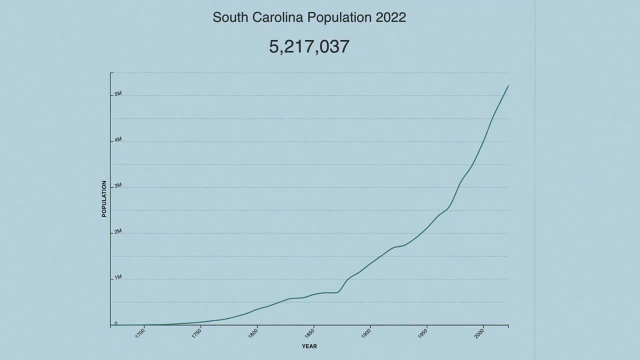 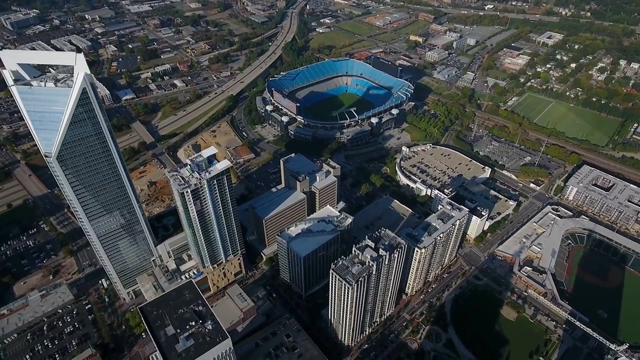 in cities like Raleigh, Charleston and Columbia too. That's because both states are growing in population and prosperity, with North Carolina adding more people but South Carolina growing at a greater percentage since 2010.. However, North Carolina's economy is still clearly ahead of its southern neighbor, with 13 Fortune 500 companies being located in. the state of North Carolina, and I'm talking about major businesses like Bank of America, Lowe's and Honeywell here, while there are no Fortune 500 companies located in South Carolina at all. The difference in economic output is even more staggering when you look at South Carolina's.